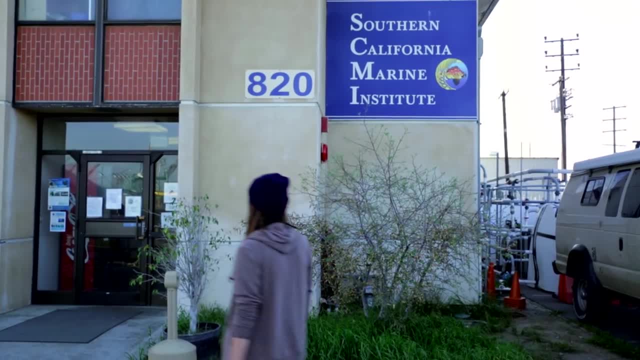 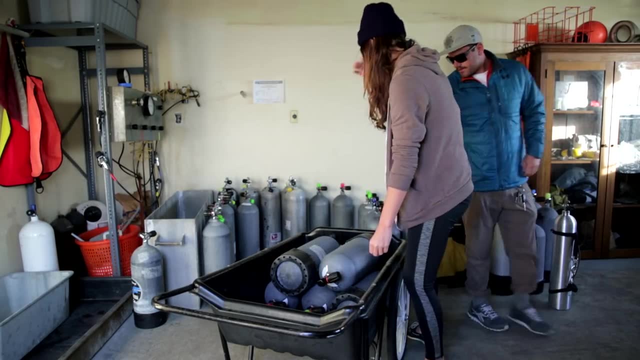 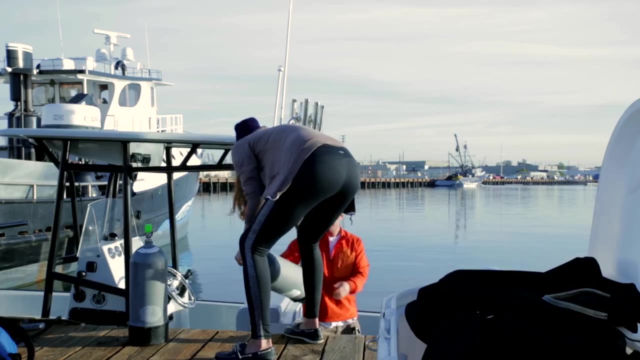 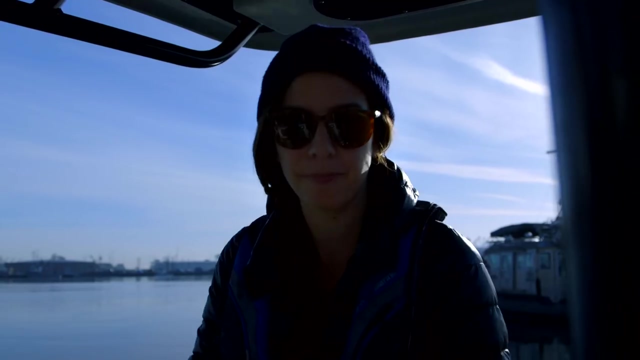 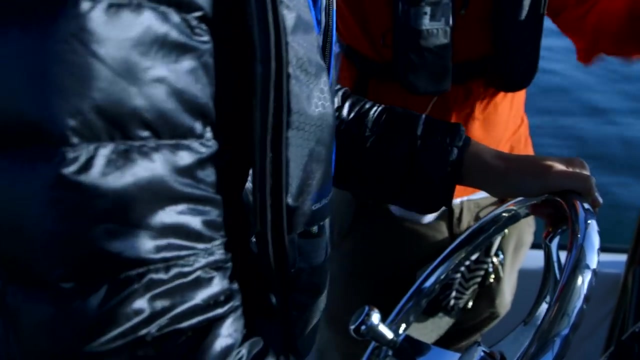 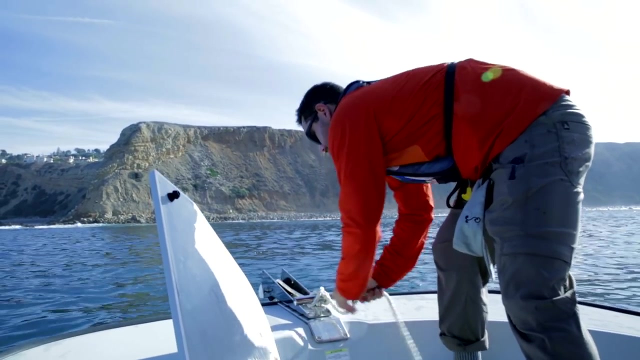 bacteria and pollutants. I work on the marine team of the Bay Foundation and basically we're working to kind of reverse those impacts and restore the natural ecosystems of the Santa Monica Bay. Ready, Ready Fingers away. On a typical dive day, we'll do three dives and each dive is in between an hour and an hour and a half. 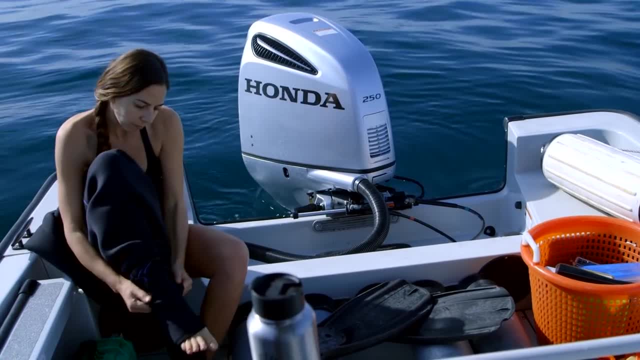 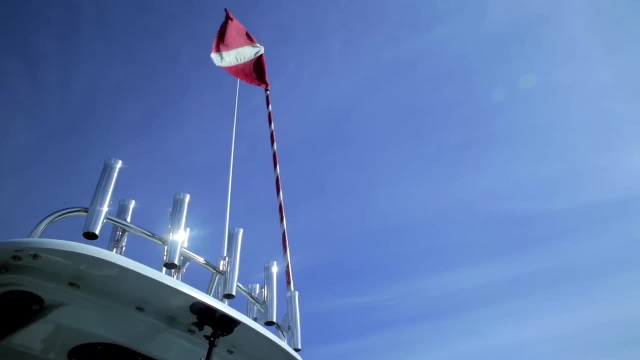 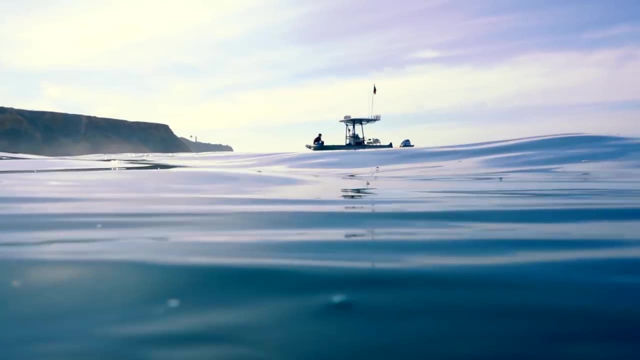 That's a lot of neoprene We have to put on all of our wetsuits, which is a lot of pieces. It's kind of cold. I love being able to see part of Earth that not many people get to see very often. 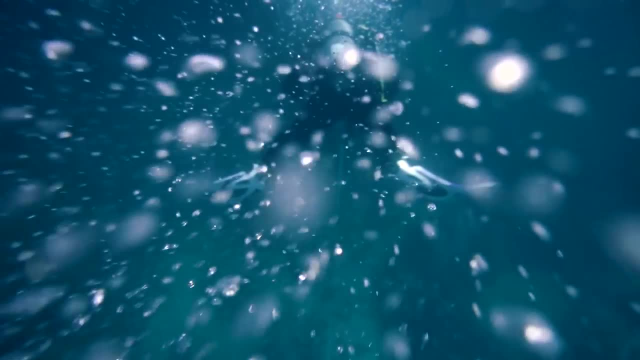 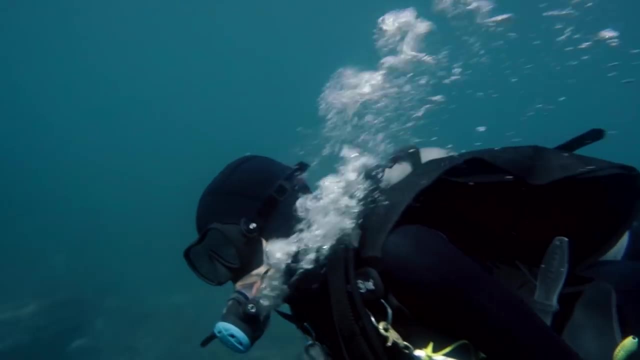 Being underwater kind of feels like being in space, because you're weightless, so you just have more space. There's no resistance on all sides of you, so you just feel like you're in a different world. almost Before we do the restoration, we look at the entire site. 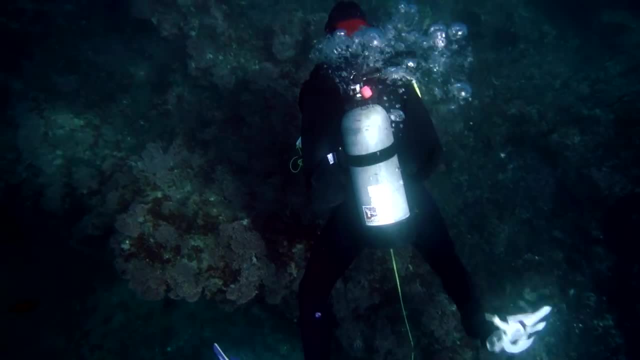 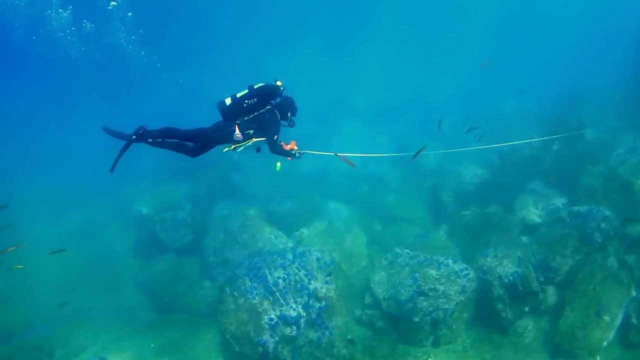 When we're down there we're looking for the density of urchins. We keep track of the amount of kelp that's already there, if there's any, and record every meter of rock and kelp and urchins that are there. 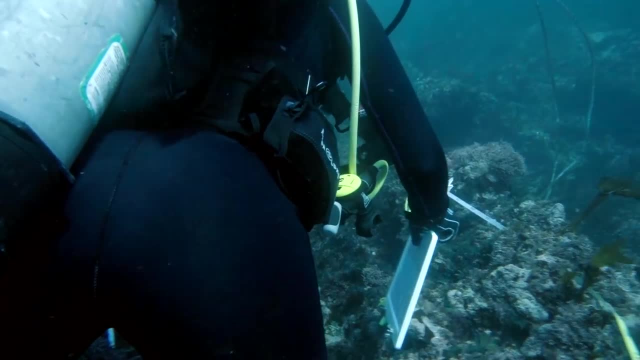 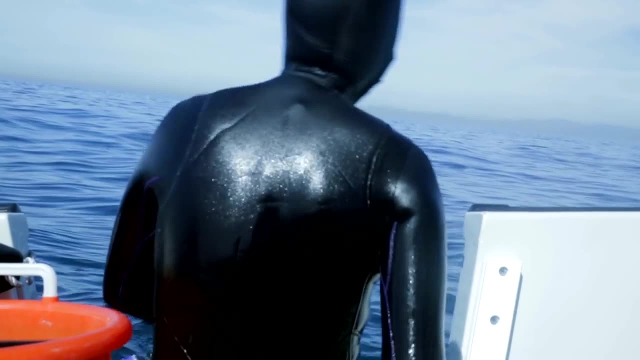 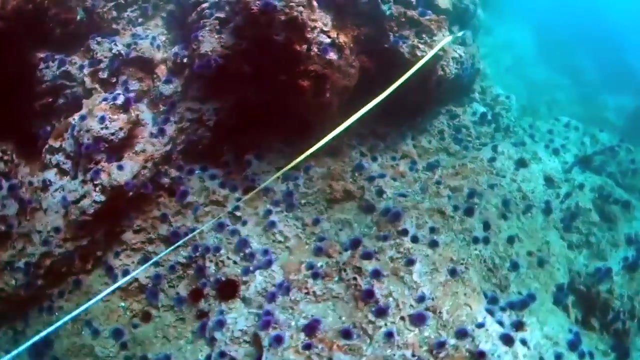 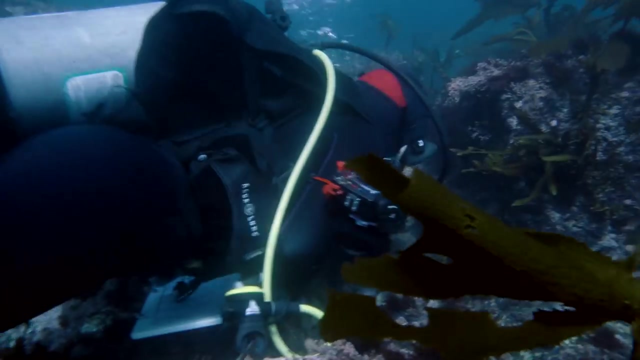 It's a lot of counting. So an urchin barren is an area where urchins have completely overpopulated a rocky reef area to the point where kelp cannot really populate that area. Kelp grows really quickly, so we're actually able to see the fruits of our labor pretty quickly. 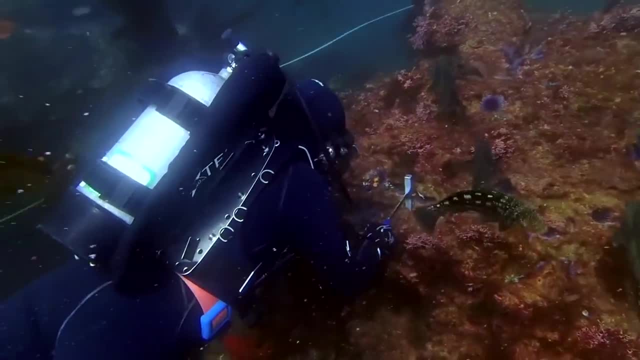 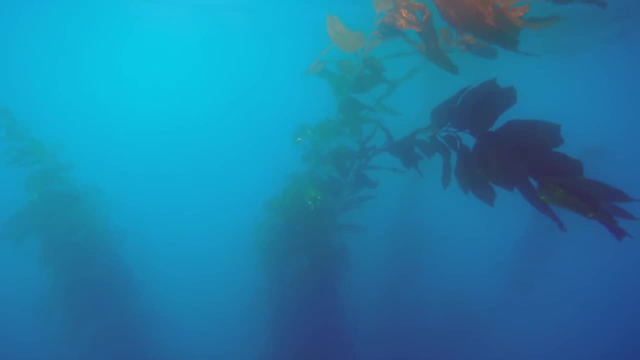 So you go in and you remove some of the urchins from this urchin barren and within two weeks there's little algae growing. And then within a month there's kelp plants. And then within six months the kelp plants have reached to the surface of the water. 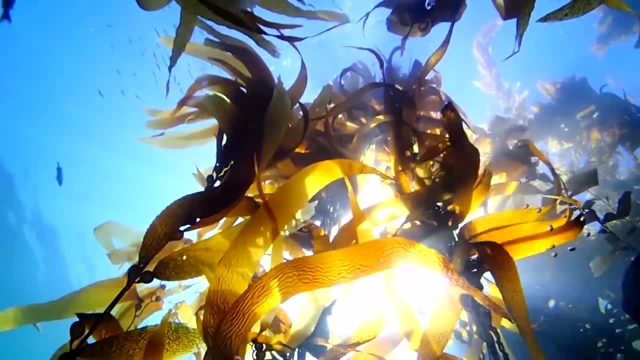 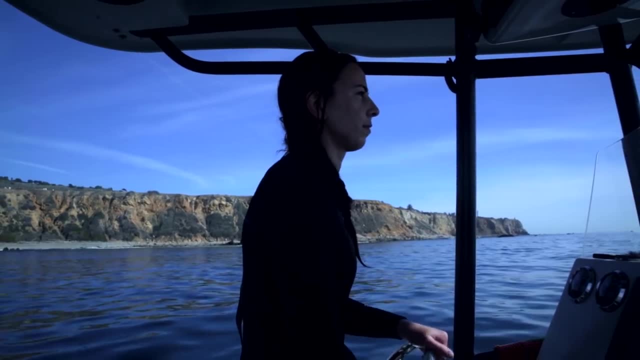 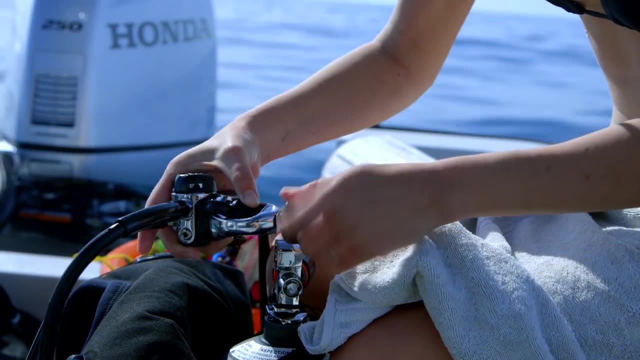 So it's kind of like watching a forest grow in front of your eyes, but underwater. The most common thing I get from people when I tell them what I do is that's what I wanted to be when I was a kid, And there's a reason that all those people didn't end up doing that, because it is a lot of hard work.